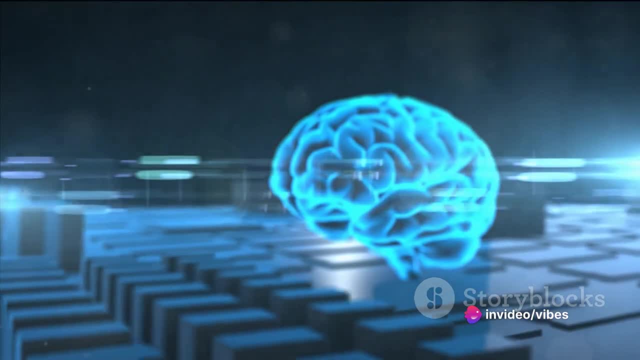 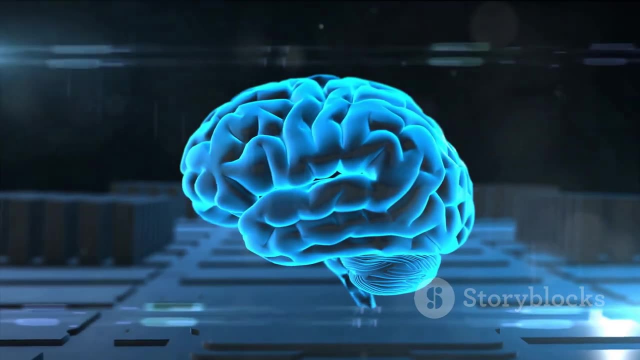 is everywhere. It's in our smartphones, helping our cameras take better photos. it's in our hospitals, aiding doctors with diagnoses. it's in our banks, predicting market trends. and it's even in our cars, enabling autonomous driving. Deep learning, a subset of 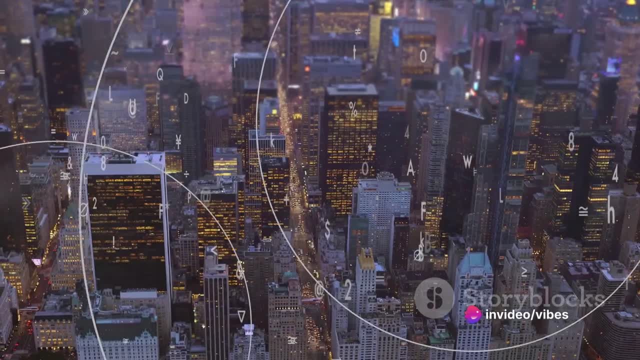 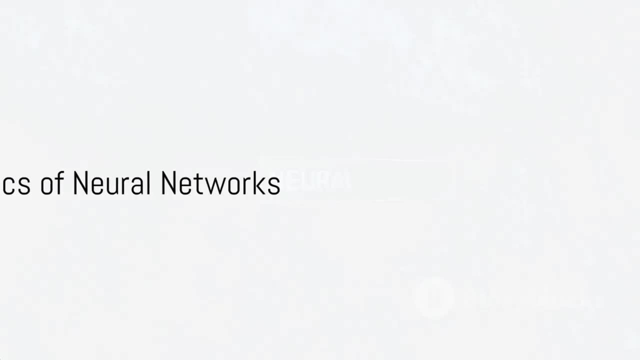 AI is transforming the world one neuron at a time. So buckle up as we dive deeper into this fascinating world of artificial neural networks and algorithms. The foundation of deep learning lies in the concept of neural networks. These fascinating neural networks are the foundation. 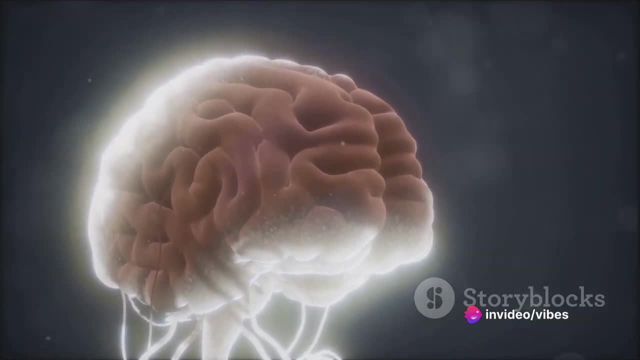 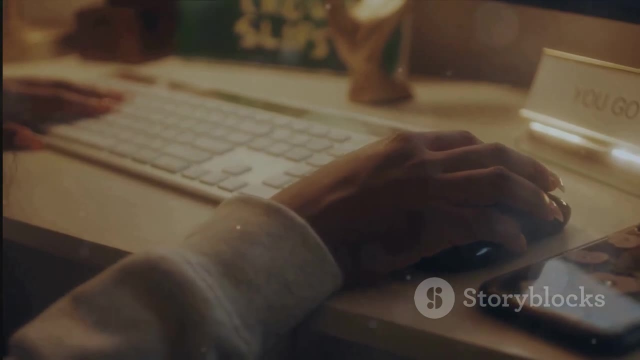 of deep learning. These fascinating neural networks are the foundation of deep learning. These fascinating constructs are designed to mimic the human brain's complex network of neurons. They're composed of layers, each containing numerous interconnected nodes or neurons. The first layer is the input layer, which receives the initial data for processing. 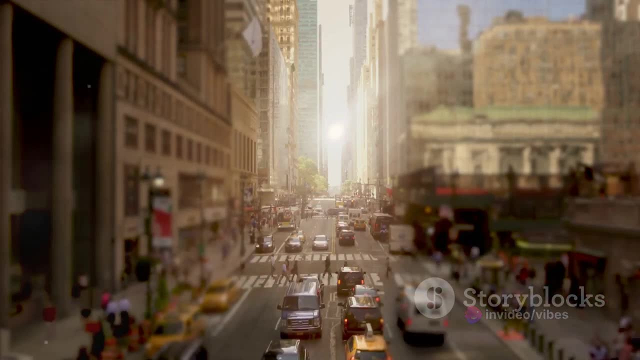 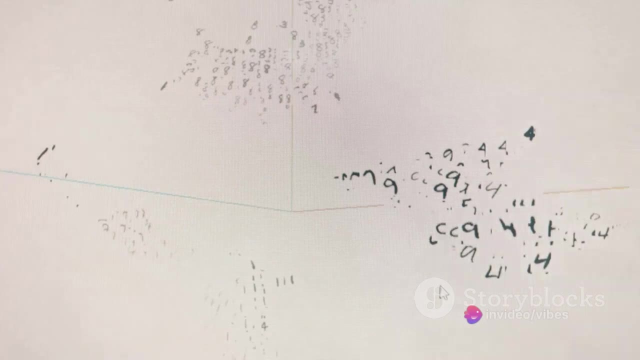 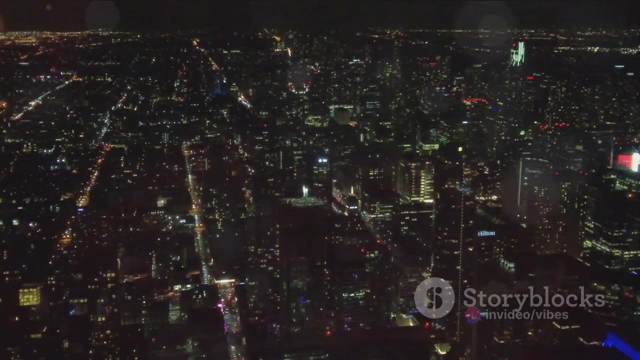 This data is then passed through one or more hidden layers. where the magic happens. Each neuron in these layers processes the incoming information, applying weights and biases, and passes it on to the next layer. The more hidden layers, deeper the network and the more complex patterns it can learn. Finally, the processed data reaches. 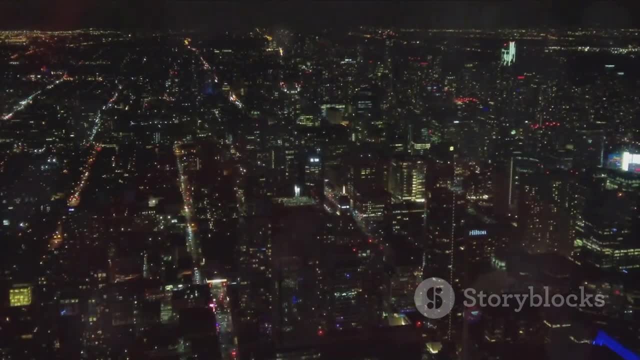 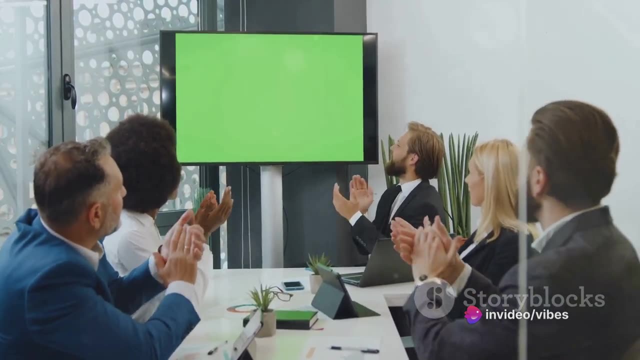 the output layer, where the network's final decision or prediction is made. Each neuron in this layer represents a possible output, and the one with the highest value is typically selected as the result. In essence, neural networks are designed to learn from data, much like how our 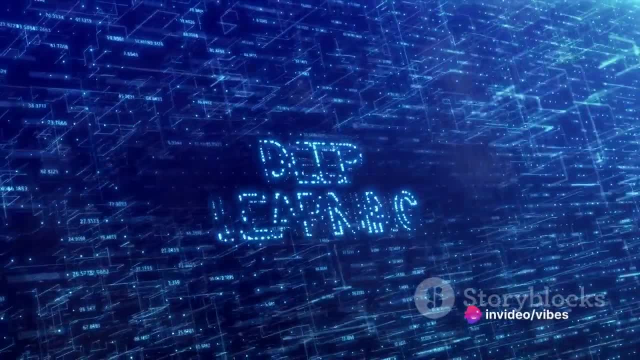 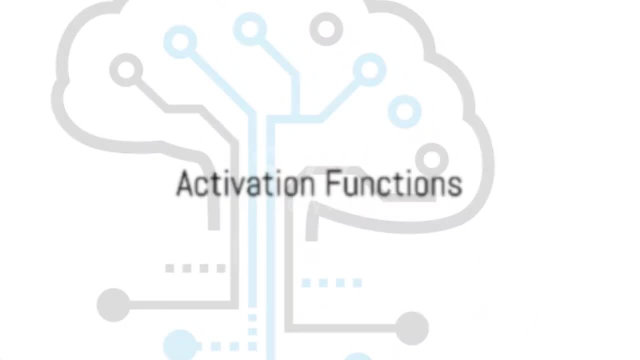 brains learn from experiences. Neural networks, the building blocks of deep learning model, the intricate workings of the human brain. Neural networks are designed to learn from data, much like how our brains learn from experiences. Now it's time to activate your understanding of activation. 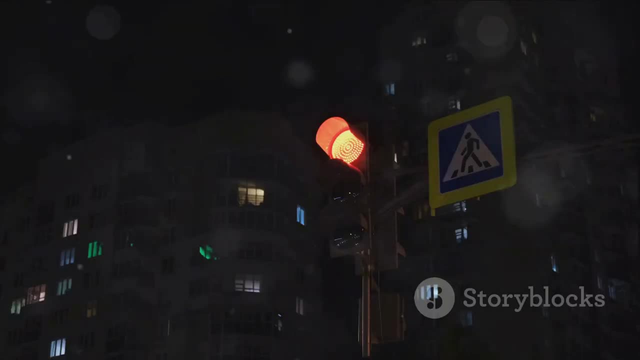 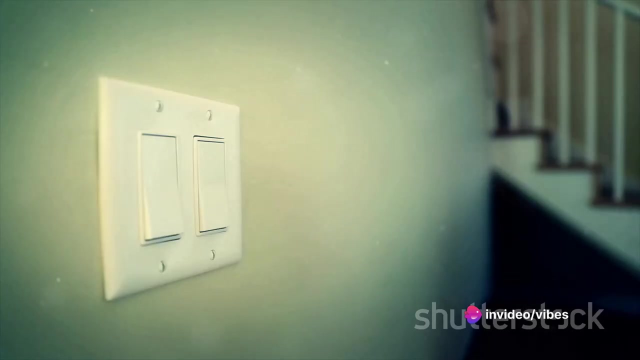 functions. Just as a light switch controls the flow of electricity, activation functions govern the transmission of information in a neural network. They're the gatekeepers determining what gets through and what doesn't. Three widely used activation functions are: ReelU, Sigmoid. 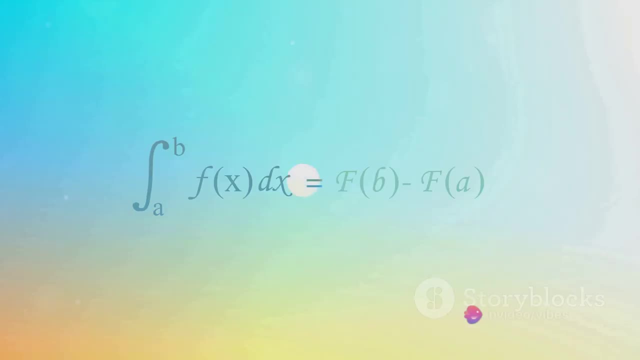 and Tan. ReelU, or rectified linear unit, is like an all-or-nothing switch. It passes positive values as they are and blocks negative ones. Sigmoid, on the other hand, is a bit more flexible. It squeezes all input values between 0 and 1, providing a probabilistic output Then. 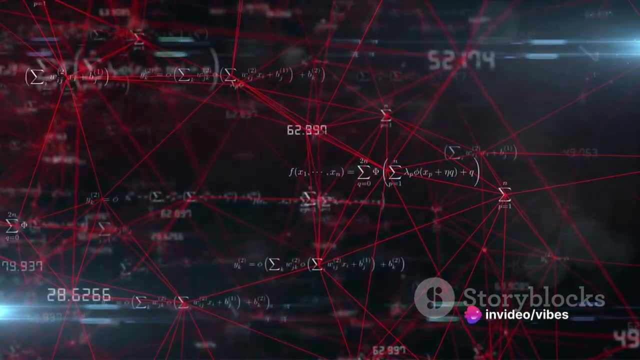 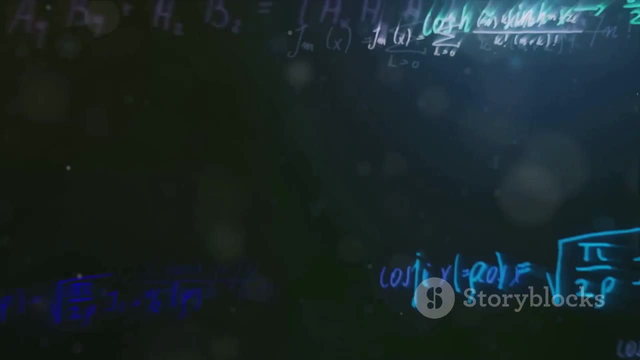 we have Tan, which is a scaled version of the Sigmoid function. It outputs values between negative 1 and 1, making it a great choice when we want to distinguish between positive and negative inputs. So what's the big deal with these functions? Well, they shape the 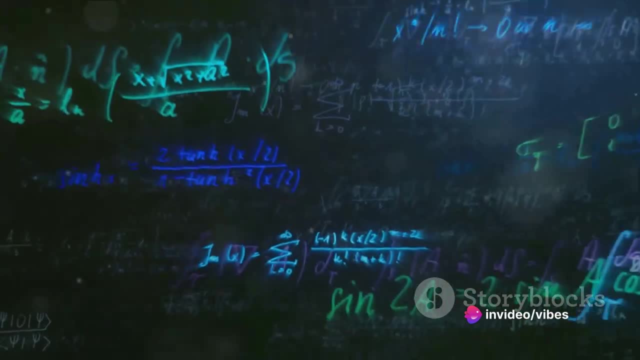 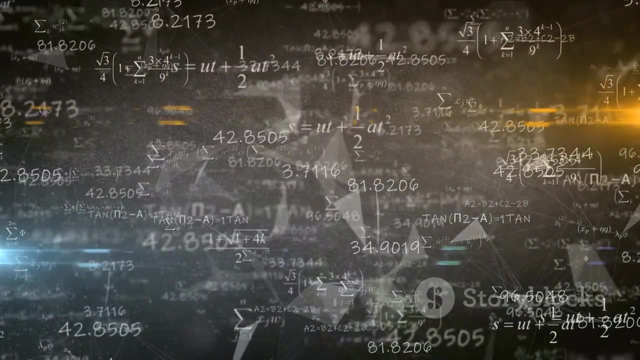 output of a neuron guiding the network's learning process. Activation functions are the unsung heroes of deep learning, making the magic of neural networks possible. Neural networks are the ones that shape the output of a neuron guiding the network's learning process. 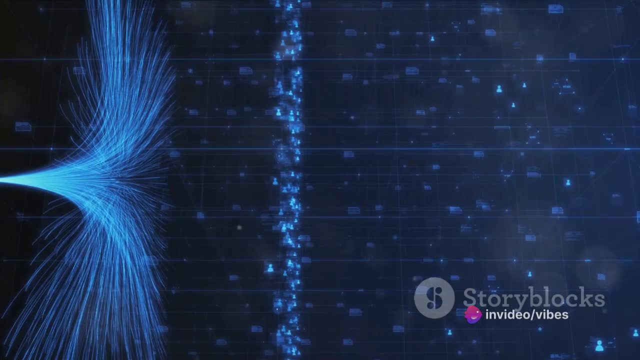 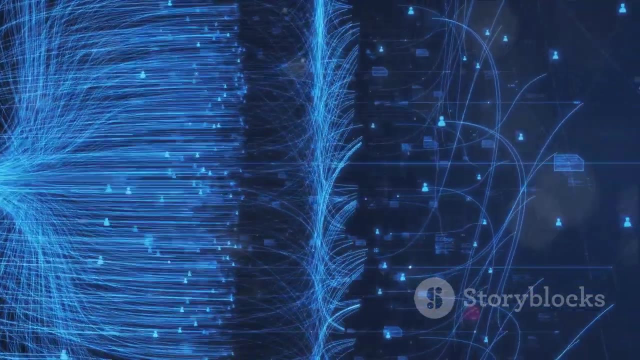 Journey through the network, with forward and backward propagation. These two processes are the heartbeats of a neural network's learning journey. Forward propagation is the network's initial guess. It's the process of moving from the input layer through the hidden layers. 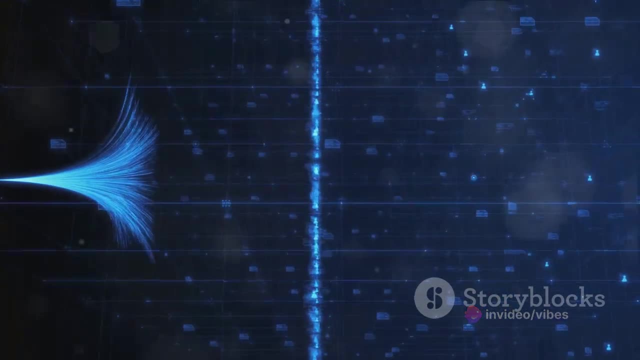 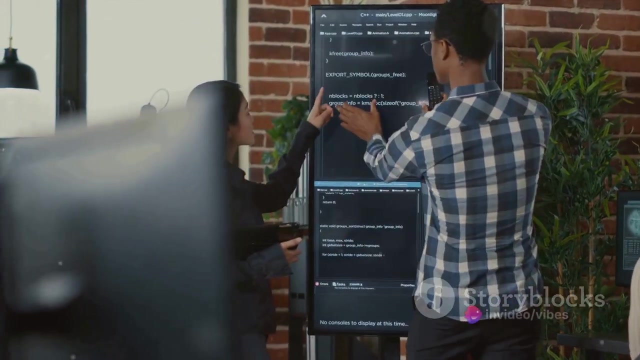 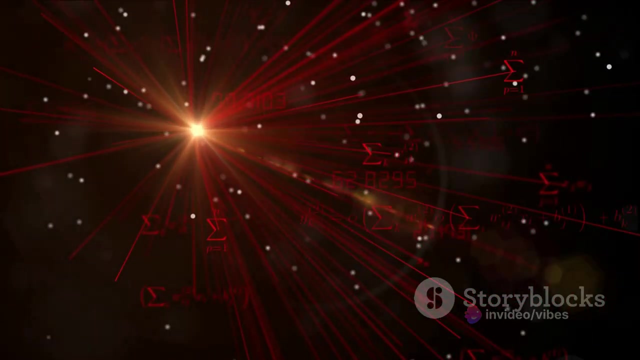 to the output layer. The network makes a prediction, but it's often wrong at first. That's where backward propagation steps in Pro-propagation. it's the process of going back through the network to adjust the weights. The network uses a cost function to measure how far off its prediction was from the actual. 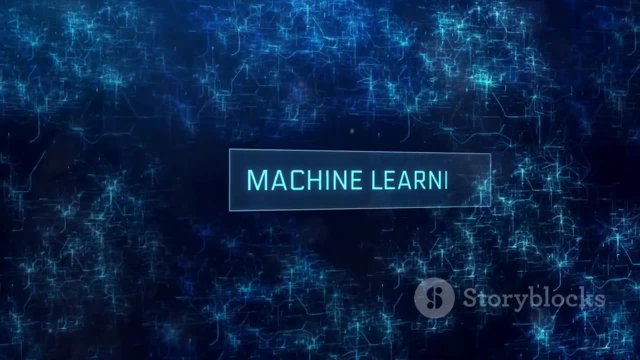 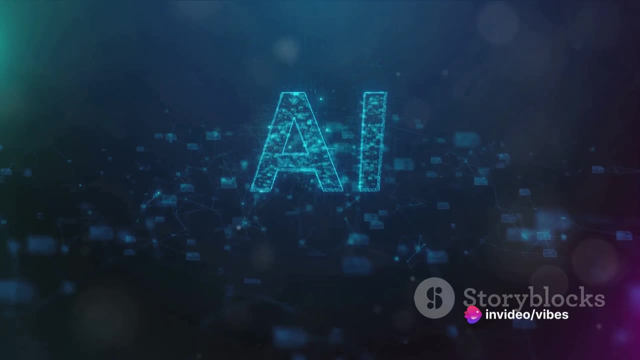 result. Then, through the magic of calculus and the chain rule, it calculates how much each weight contributed to the error. These weights are then adjusted, reducing the error for future predictions. This cycle of forward and backward propagation continues, refining the network's ability. 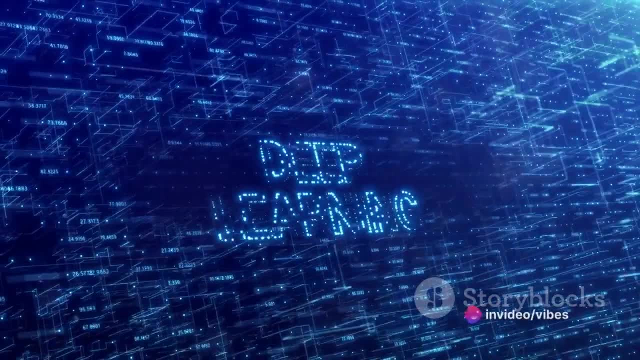 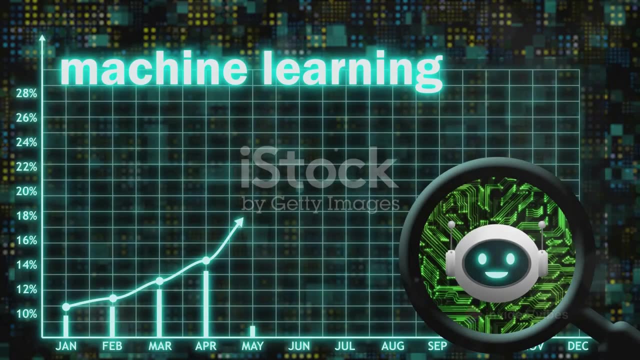 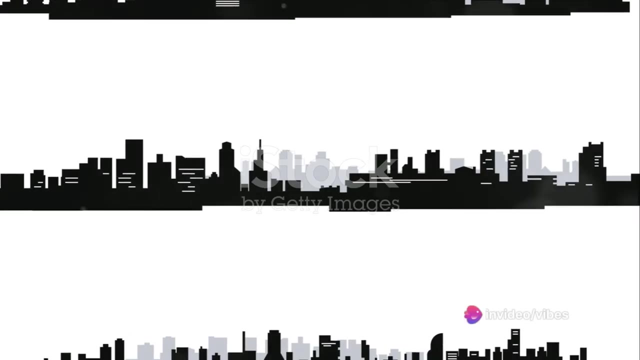 to predict accurately. techniques enable a network to learn from errors and refine its predictions. meet the unsung heroes of deep learning, the optimizers. these are the algorithms that steer the learning process, guiding our neural networks to the best possible solutions. at the heart of optimization, we find the 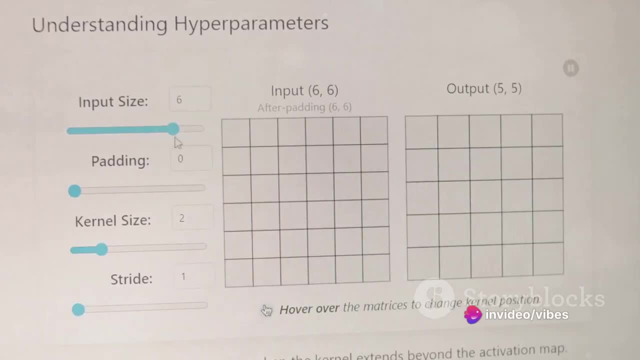 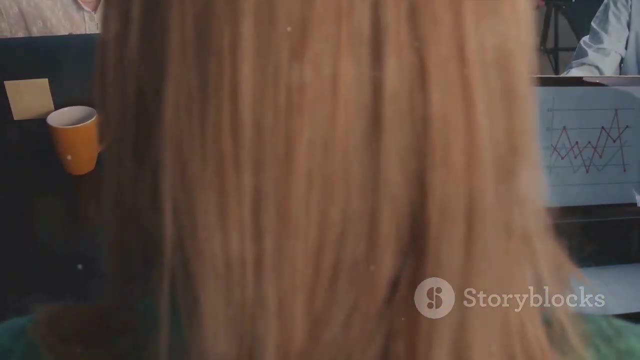 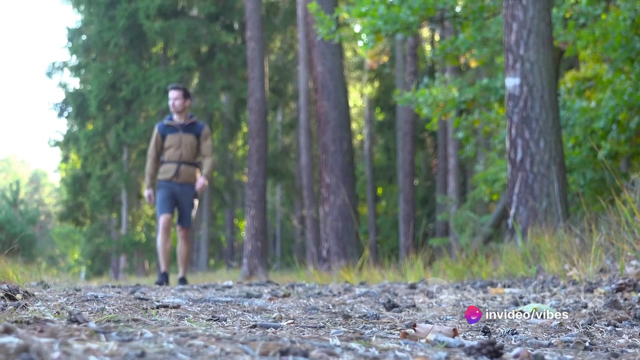 loss function. this is the measure of how far our model's predictions are from the actual results. the optimizer's job: minimize this loss. consider gradient descent, one of the most basic yet powerful optimizers. it's like a hiker trying to find the lowest point in a valley, taking steps. 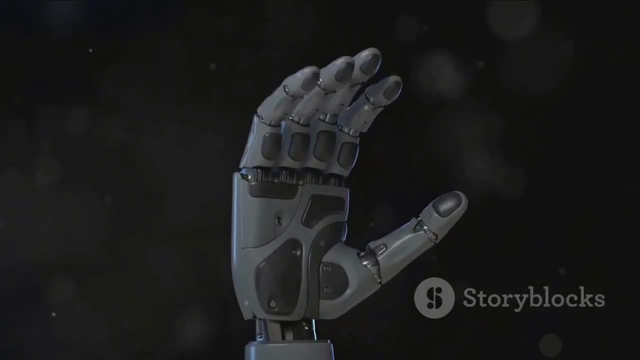 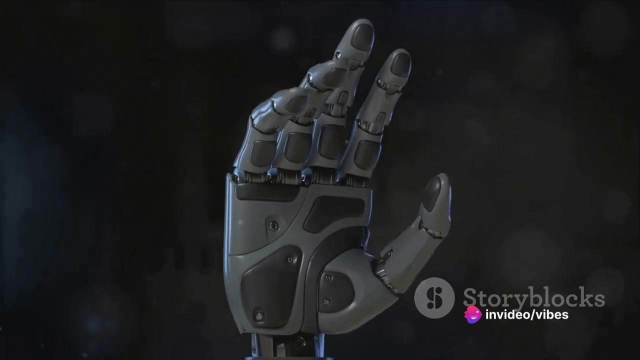 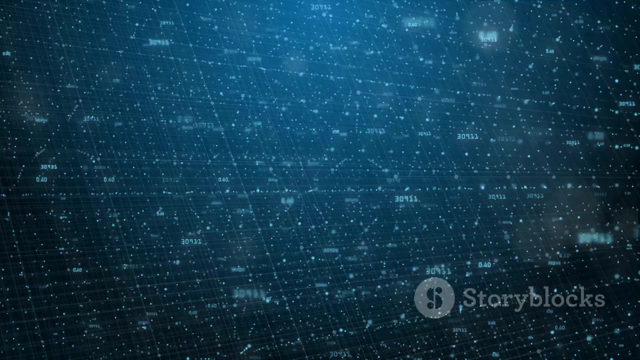 proportional to the steepness of the slope. it iteratively adjusts the model's parameters, reducing the loss function until it finds the minimum. then there's adam, short for adaptive moment estimation. it's a bit more sophisticated, combining the perks of two other optimizers: momentum and rms prop. adam adapts the learning rate for each weight in the network. 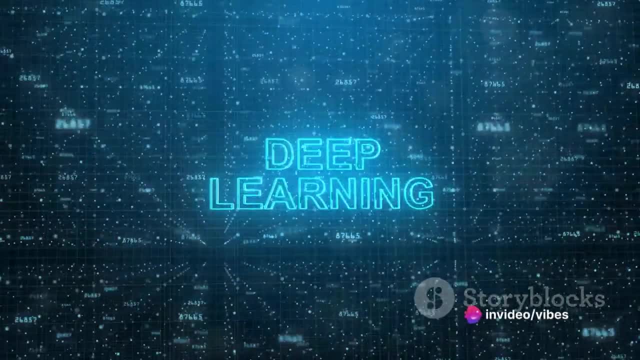 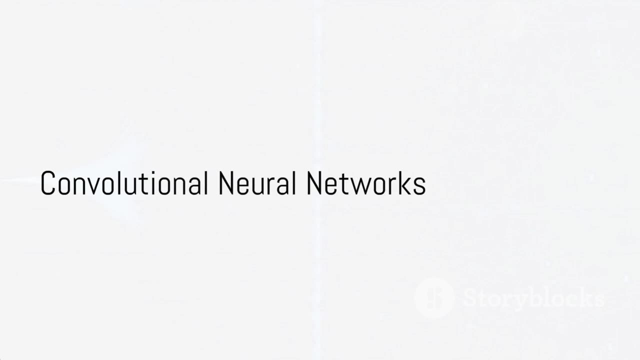 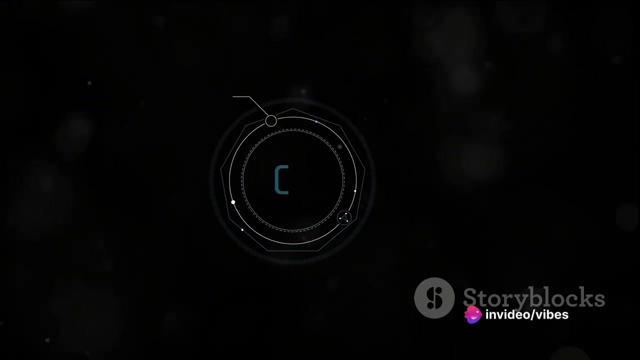 providing a more precise and efficient optimization. optimizers fine-tune the learning process, driving the network towards accurate predictions. ever wondered how facebook recognizes your face? meet convolutional neural networks. these are a special kind of neural network designed specifically for processing visual data. picture them as the eyes of artificial intelligence, allowing machines to see and 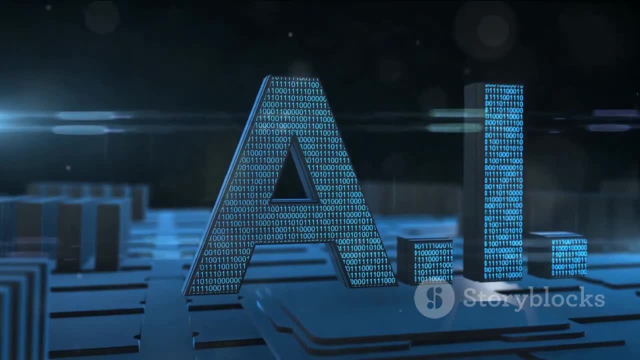 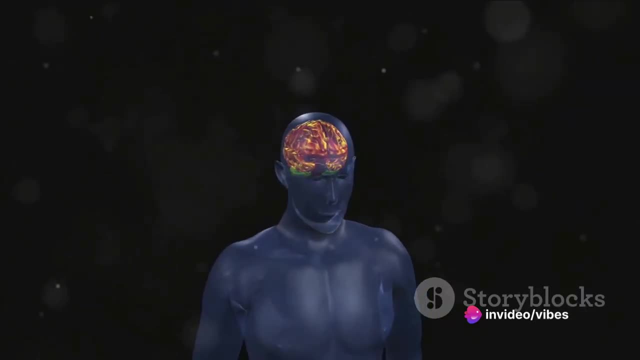 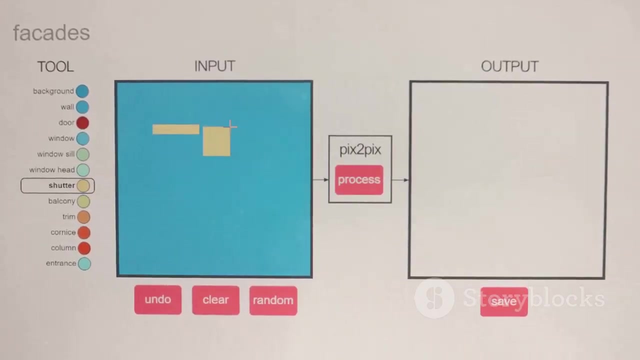 understand images and videos. the structure of cnn's is inspired by the human visual cortex, the part of our brain responsible for interpreting what we see and what we see. they consist of multiple layers, each designed to detect different features in an image. while the initial layers might identify simple patterns like lines and edges, the deeper 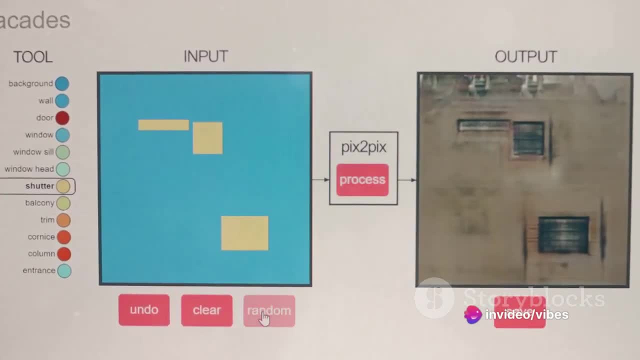 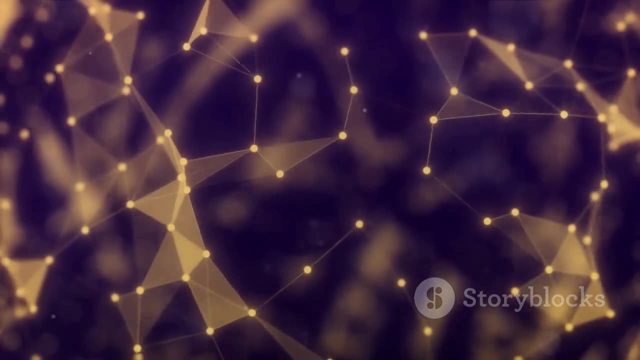 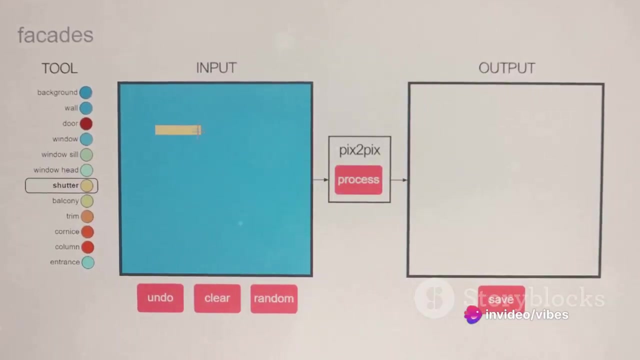 layers recognize more complex structures like shapes and objects. what really sets cnn's apart is their ability to maintain spatial relationships. they don't just see individual pixels. they understand how these pixels relate to each other to form a coherent picture. this makes them incredibly powerful in tasks like image and video recognition. they're able to see individual pixels. 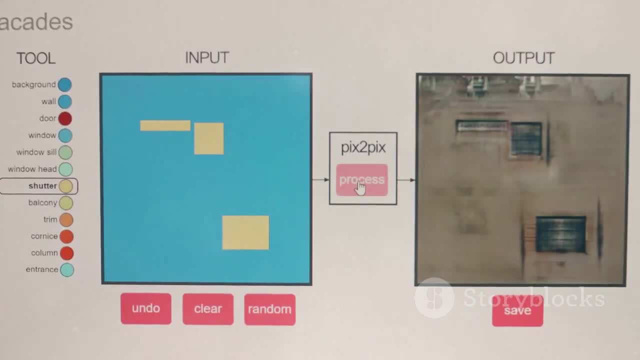 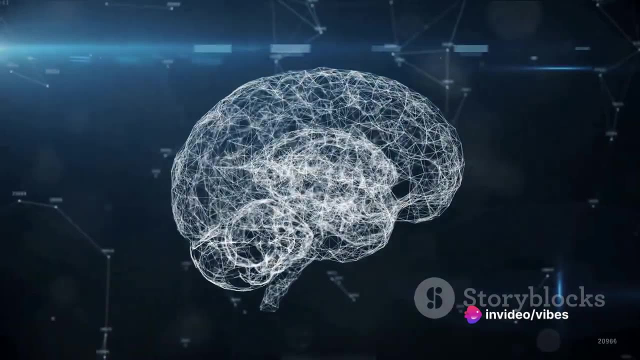 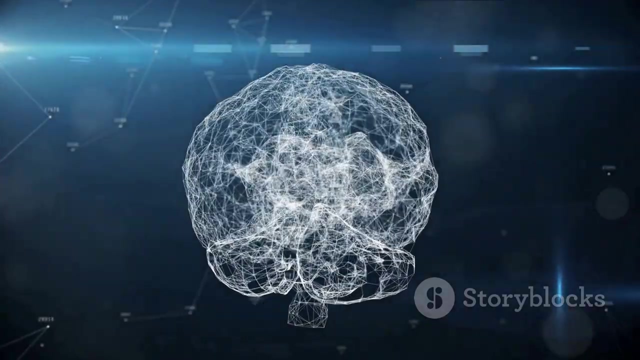 cnn's, the visionaries of deep learning, allow machines to see and interpret visual data. can machines remember? with recurrent neural networks they can. recurrent neural networks, often referred to as rnns, are a unique breed of artificial neural networks. unlike their counterparts, rnns have a sense of memory. they achieve this by incorporating loops in their 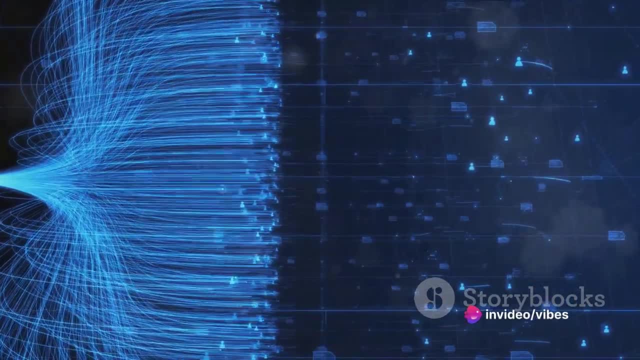 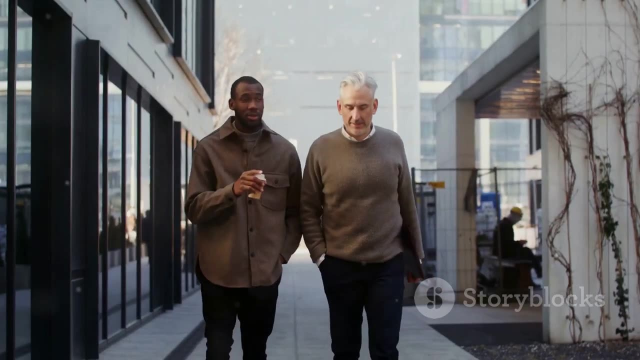 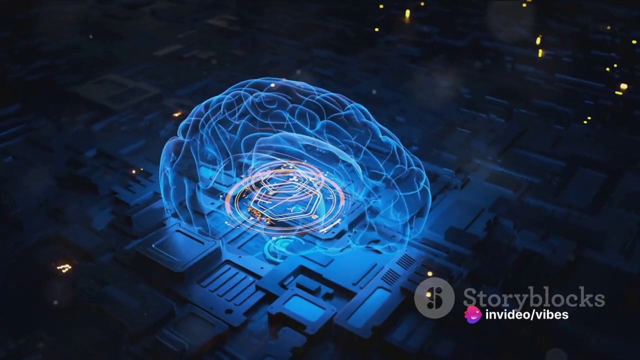 structure allowing information to persist from one step in the sequence to the next. this makes them ideal for tasks that involve sequential data like text and speech. imagine having a conversation and forgetting the previous sentence every time you hear a new one. sounds impractical, right, that's where rnns come in. 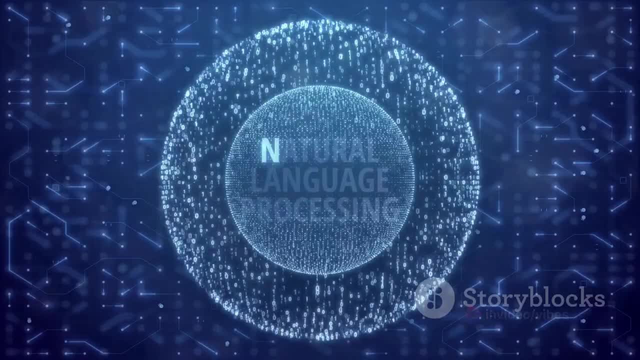 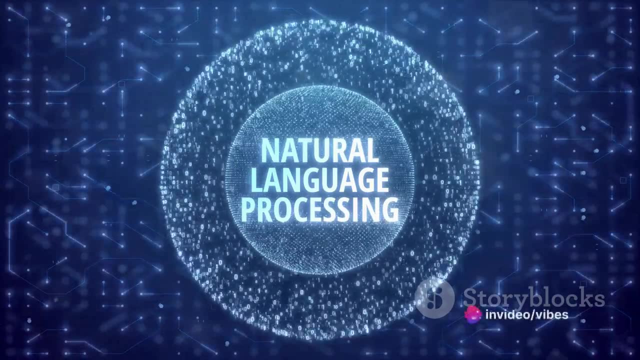 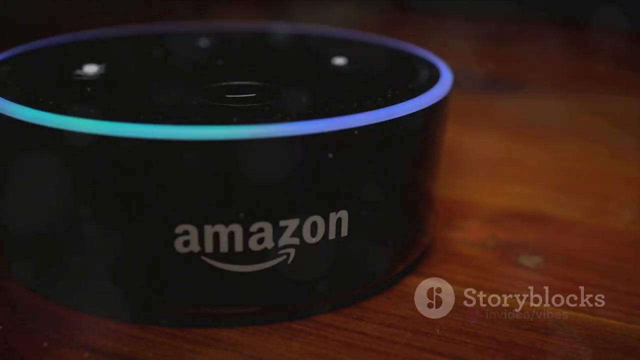 they remember the past and use this context to understand the present. this ability to process sequences makes rnns versatile. they're used in everything from language translation to speech recognition, and even in generating creative content like music and poetry. so the next time you ask your smart speaker a question, remember it's the recurrent. 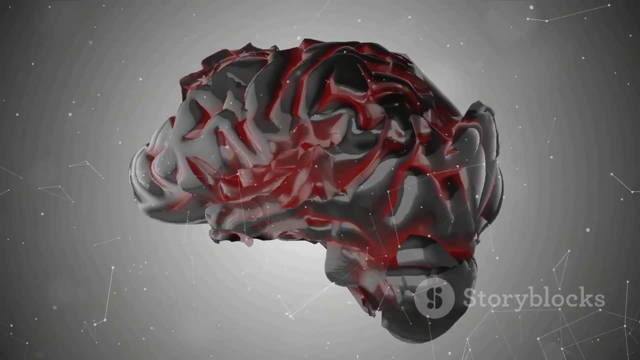 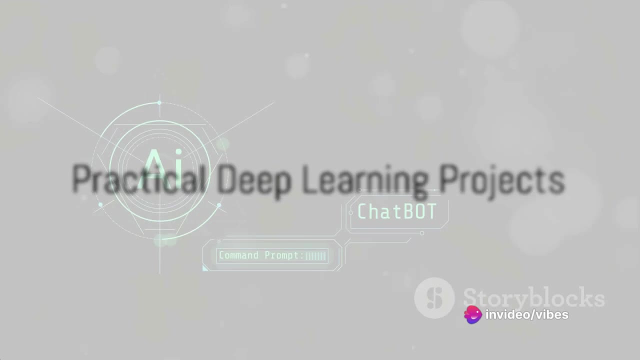 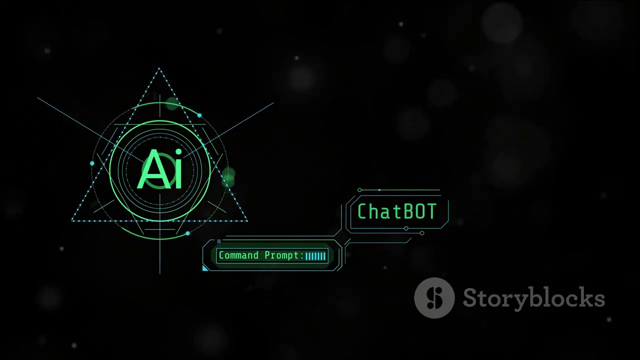 neural networks that make it possible. RNs give machines a memory enabling them to understand and generate language. Now let's bring all these concepts together with some real-world deep learning projects. Imagine a world where machines can understand and interpret human language, where they can. 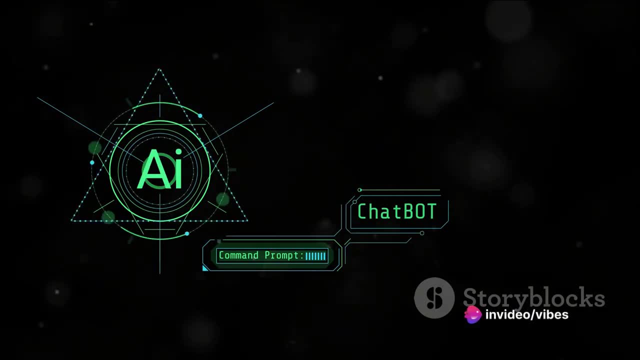 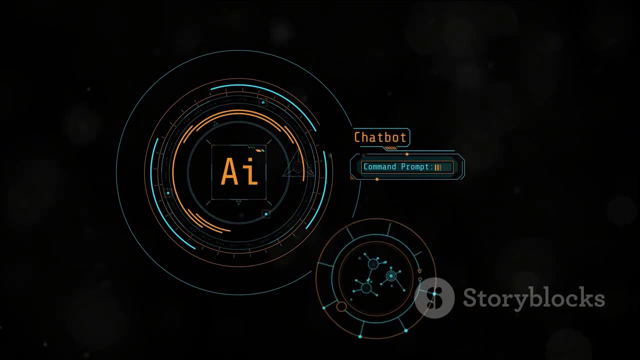 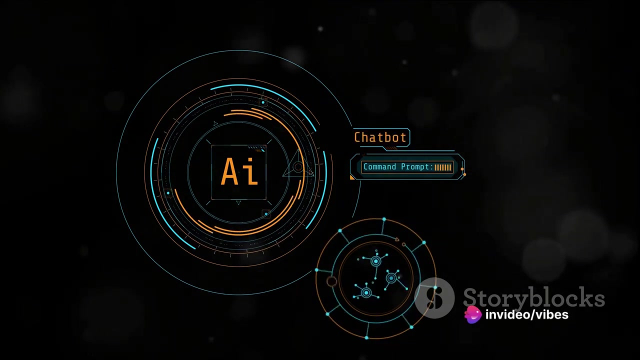 recognize objects and people and even predict future events. Well, this is no longer a figment of our imagination, it's reality. and it's all thanks to deep learning. One practical application of deep learning is in natural language processing. An impressive example is the development of chatbots that can understand and respond to. 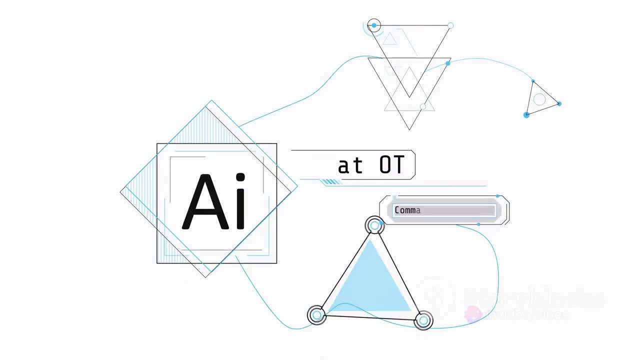 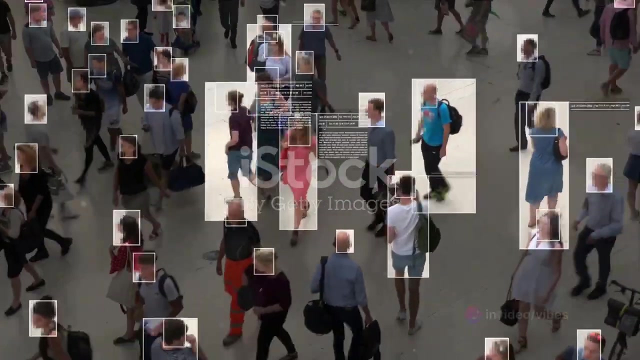 human language in a way that feels almost human. By using recurrent neural networks, these chatbots can understand context, sentiment and even sarcasm, making them more engaging and useful than ever before. Then we have object recognition, a key component of many modern technologies from self-driving. 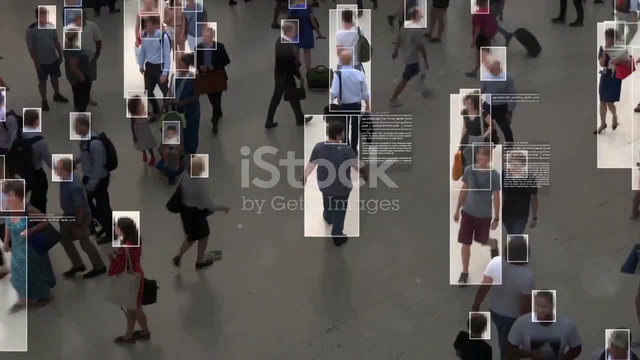 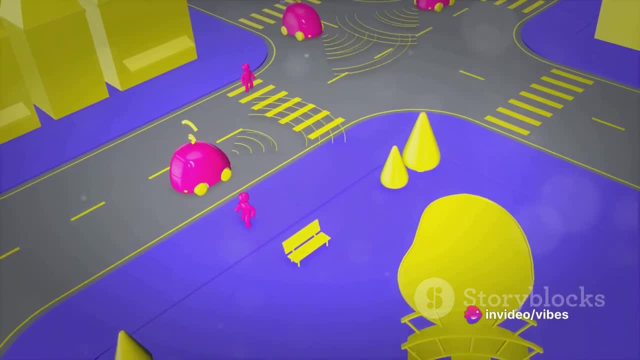 cars that need to identify pedestrians, to cars that need to identify pedestrians to other vehicles. to social media platforms that automatically tag you and your friends in photos. Deep learning is at the heart of these technologies: Convolutional neural networks with their ability to recognize patterns and details. 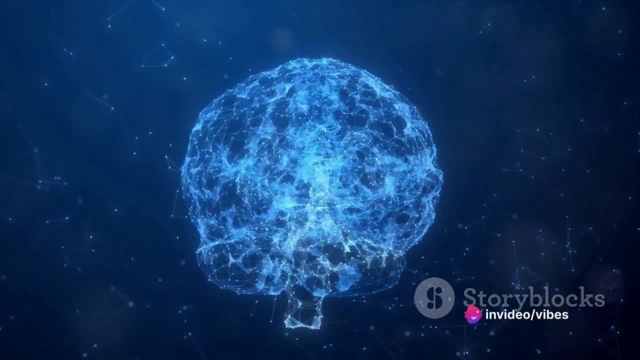 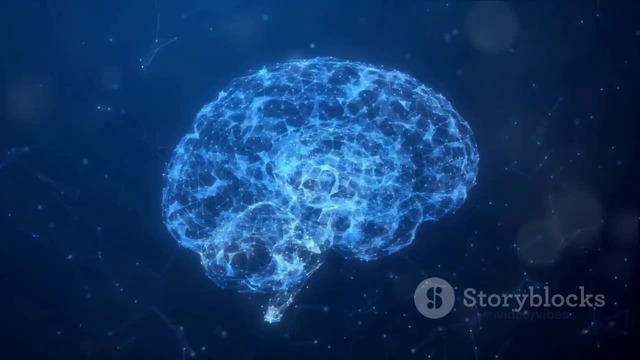 are the heroes behind these feats. Let's not forget about predictive analytics, another area where deep learning shines. By analyzing patterns in vast amounts of data, deep learning models can predict future trends and events with astonishing accuracy. This is particularly important for deep learning, because deep learning models can predict future. 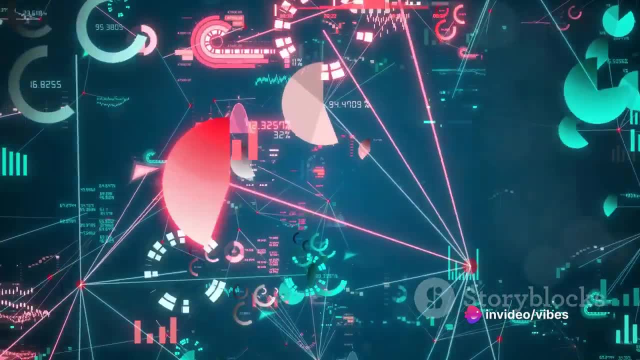 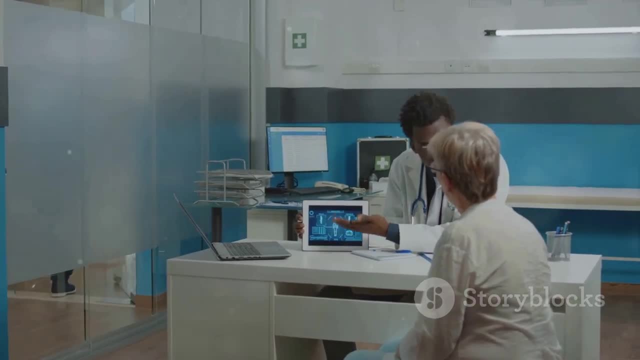 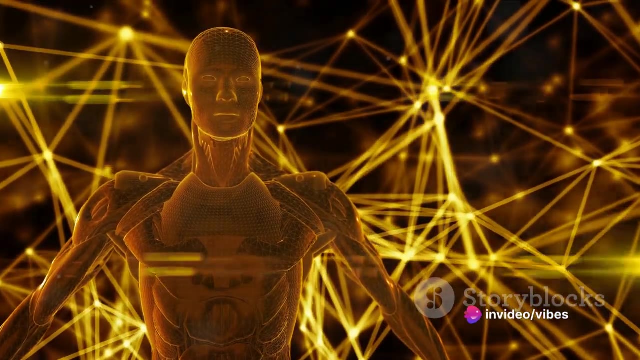 trends and events with astonishing accuracy. This is particularly useful in industries like finance, where predicting market trends can mean the difference between profit and loss. Deep learning also plays a crucial role in healthcare, helping doctors diagnose diseases more accurately and quickly. By analyzing medical images, deep learning models can detect anomalies that might be. 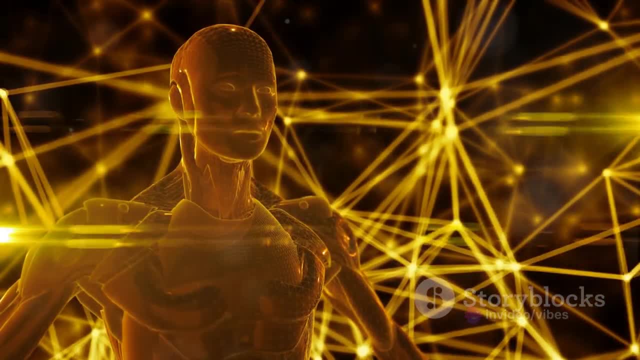 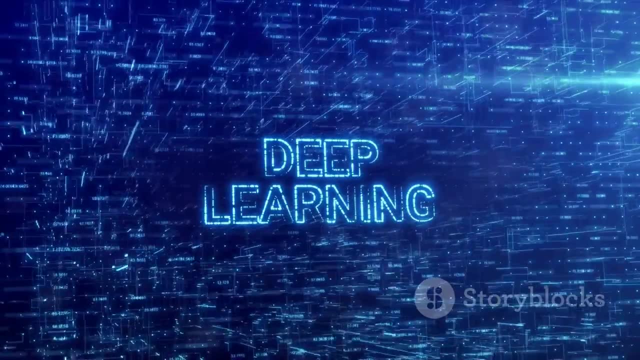 missed by the human eye, thereby improving patient outcomes. And these are just a handful of examples. The possibilities are endless, limited only by our imagination and the data available to us. So as we delve deeper into the world of deep learning, remember this: 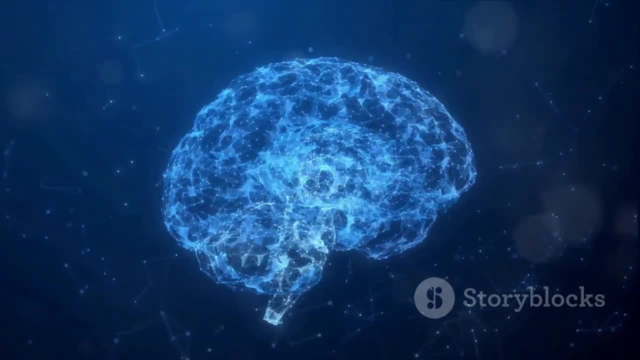 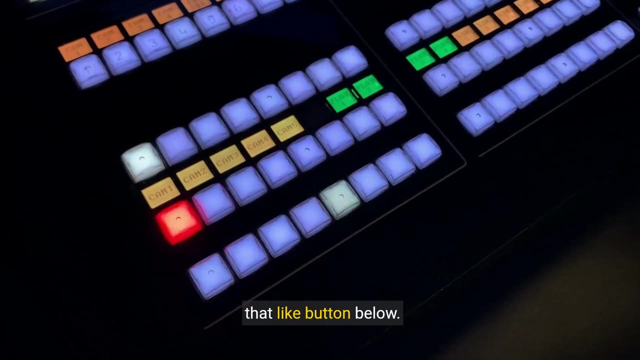 Deep learning isn't just theory. it's a practical tool that's transforming industries and lives every day. Hey there, If you're enjoying this video, don't forget to hit that like button below. Sharing is caring. Spread the fun by clicking on the share button with your friends.